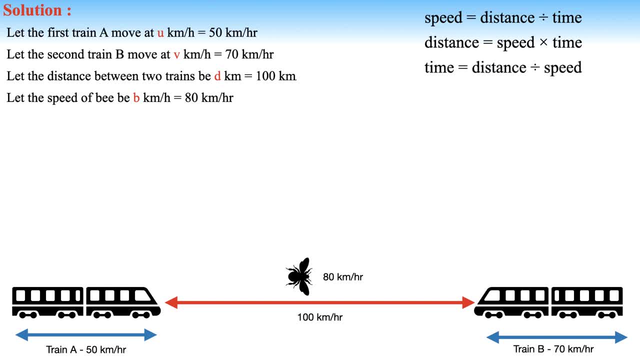 rearranged in three ways. in order to calculate speed, the formula becomes: speed equals distance divided by time. to find distance: distance equals speed multiplied with time. to calculate time, time equals distance divided by speed. to calculate one of the variables- speed, distance or time- we need the other two. therefore. 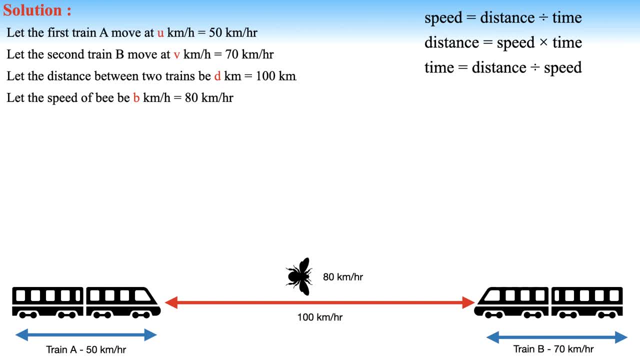 the time taken by trains to collide in this puzzle equals distance divided by speed. here, distance is d and speed is sum of speed of train a and train b, which is u plus v. hence, time taken by trains to collide equals d divided by u plus v. now, putting all the known values into the above equation, 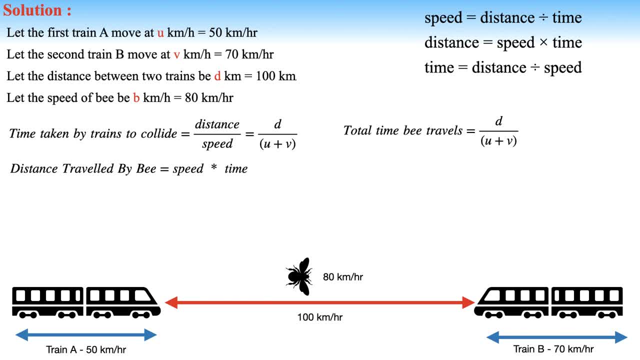 we get. so we know that u equals 50 kilometers per hour, v equals 70 kilometers per hour, d equals 100 kilometers and b equals 80 kilometers per hour. therefore, the total distance traveled by b, that is, distance equals speed multiplied with time. we know that speed of b is 80 kilometers per hour. 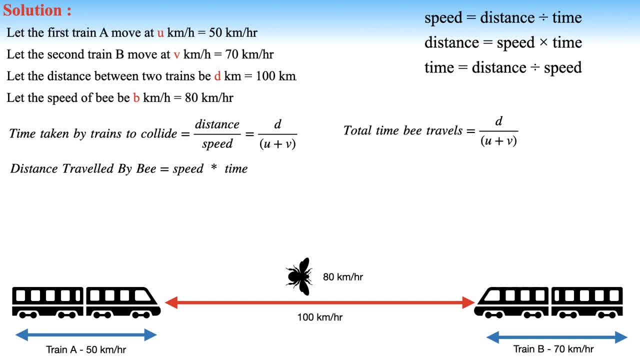 and total time b travels is d divided by u plus v. after substituting the equation becomes: distance equals b multiplied with d divided by u plus v. substituting the values of b, d, u and v, equation becomes 80 times 100. divided by 50 plus 70. after solving it results in approximately 66.67. 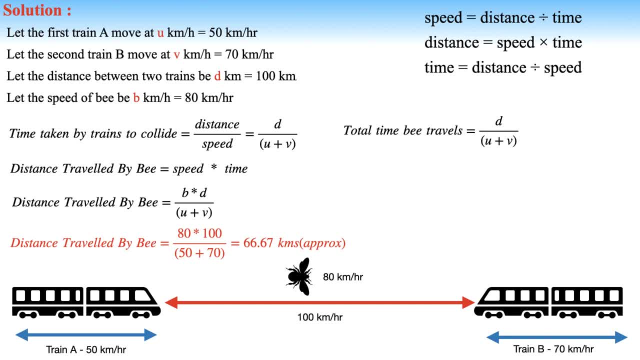 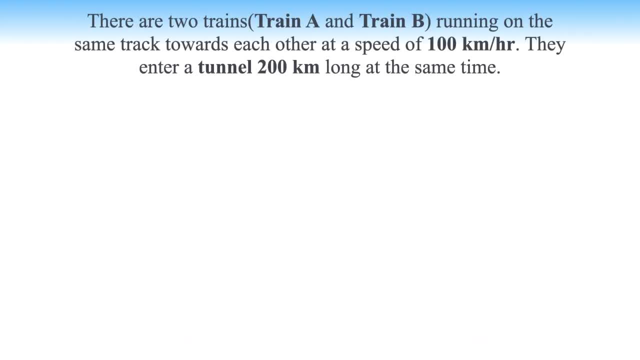 kilometers. thus total distance traveled by b is 66.67 kilometers. i am sharing one more similar puzzle. try to solve this by yourself before checking. the solution puzzle states that there are two trains, say train a and train b, running on the same track towards each other at a speed of 100 kilometers per hour. they enter a tunnel 200 kilometers long at the. 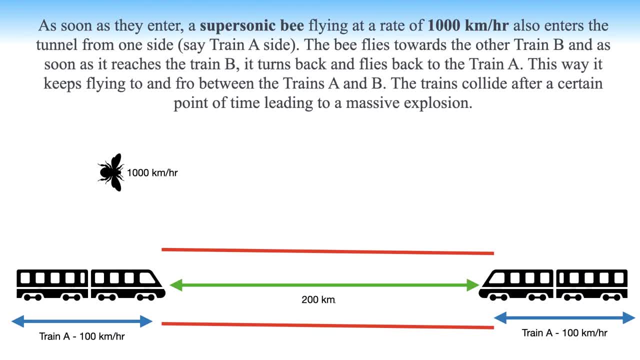 same time they enter a tunnel 200 kilometers long. at the same time they enter a tunnel 200 kilometers athan them. as soon as they enter, a supersonic b flying at a rate of thousand kilometers per hour, also enters the tunnel from one side, say train a side, the b flies towards the other train b. 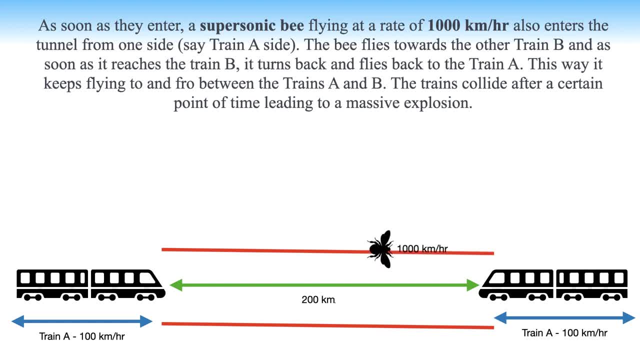 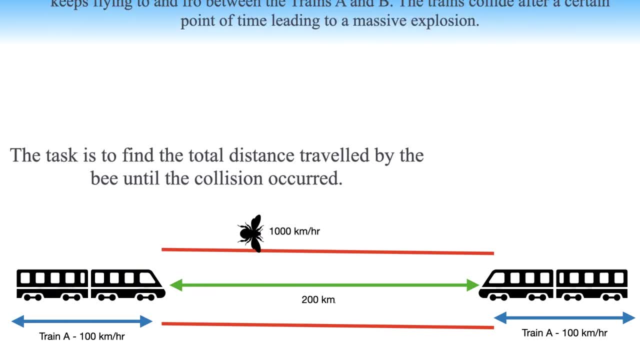 and as soon as it reaches the train b, it turns back and flies back to the train a. this way it keeps flying to and fro between the trains a and b. the trains collide after a certain point of time due to a massive match in the american air traffic. the train b and female two go to one side and the true two, Otus 준 ui, skydive to the other side, trying to climb the point of a certain point in time, leading to a massiveண. 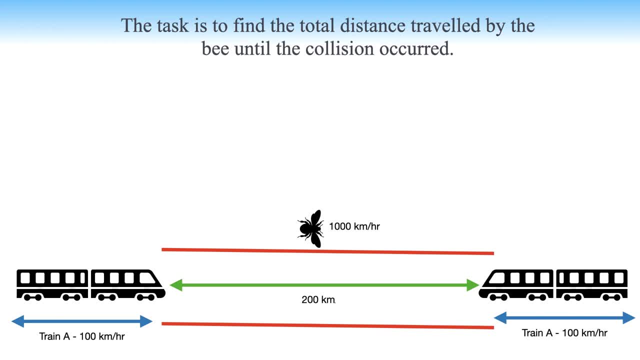 explosive explosion. The task is to find the total distance travelled by the bee until the collision occurred. Let me explain the solution now. This puzzle can be solved with the help of basic physics and observation. We know that speed of train A and train B equals 100 km per hour. Length: 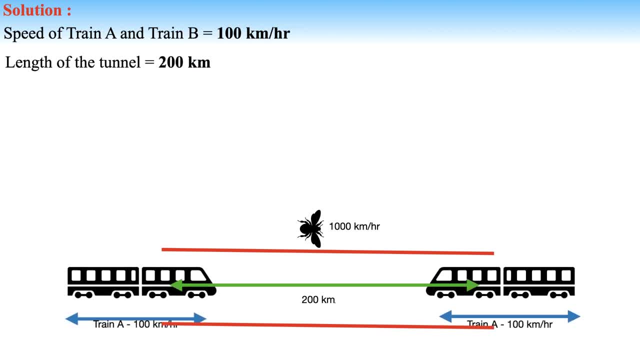 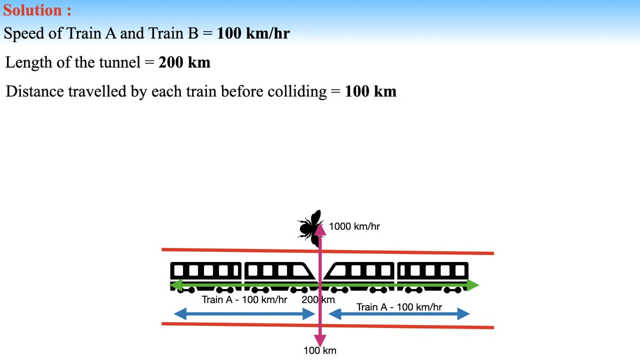 of the tunnel equals 200 km, Since both the trains are travelling at the same speed. hence they must have travelled equal distance before colliding, which means that they must have collided at the off way of the tunnel. Therefore, distance travelled by each train before colliding. 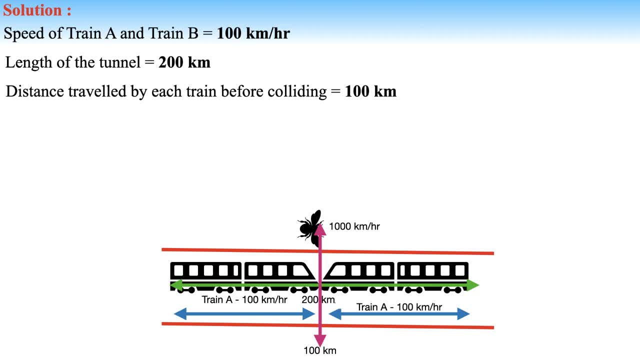 equals 100 km, Because the length of the tunnel is 200 km and time taken by each train to travel 100 km and collide equals distance divided by speed, which is equal to 100, by 100, which is equal to 1 hour. Therefore, the bee must have 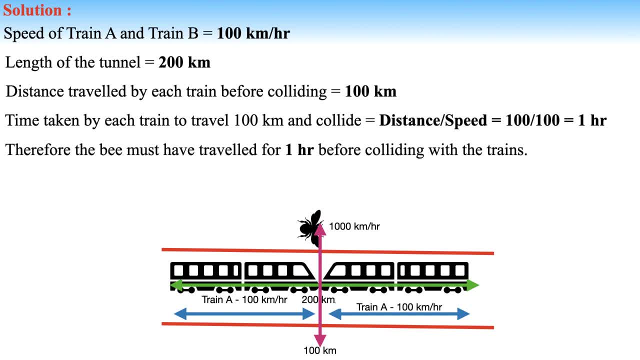 travelled for 1 hour before colliding with the trains. Hence, distance travelled by the bee in 1 hour before colliding equals speed multiplied with time, which is equal to 1000, multiplied with 1, which is equal to 1000 km. Thus, total distance travelled by bee until the collision occurred is 1000 km. 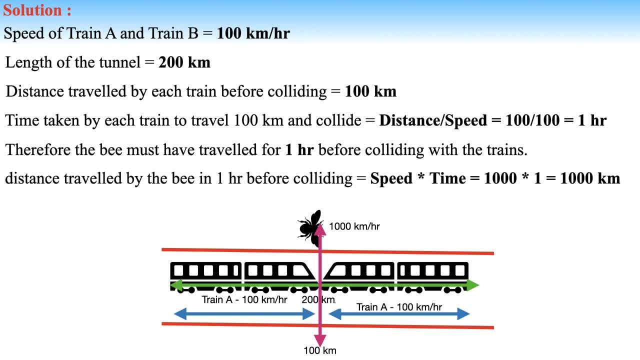 By following these simple steps, we can solve these kind of puzzles accurately in less time. That's all for this video. Let me know if you have any questions. I will try to address as soon as possible. Thanks for watching. Let's meet in the next video with one more. interesting puzzle, Thank you.